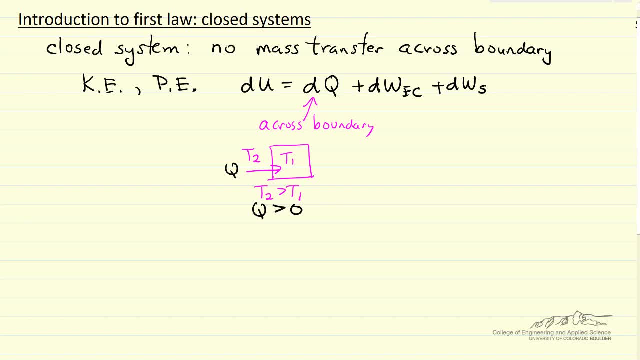 Adding energy to the system. it's positive For expansion, compression work. what we're looking at is where we have, for example, a piston cylinder arrangement and say we have a gas here and we're pushing down this piston, So we're doing work by pushing down. 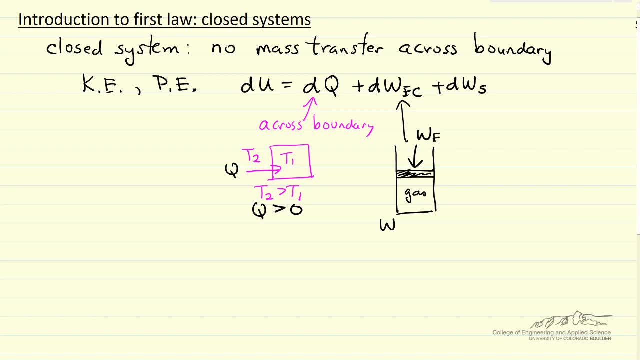 So in that case- this is expansion. compression work works greater than zero. the way I've drawn it Again, we're adding energy. Shaft work would mean, for example, we had a system with an impeller inside and this impeller is rotating. 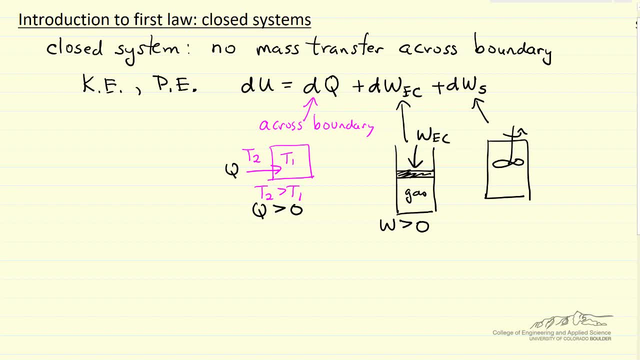 Adding energy to the fluid inside the system. Again the work, the shaft work, would be positive. We're adding energy to the system. Now, if we look at the integrated form of the first law, where delta U change in internal energy between initial and the final state, 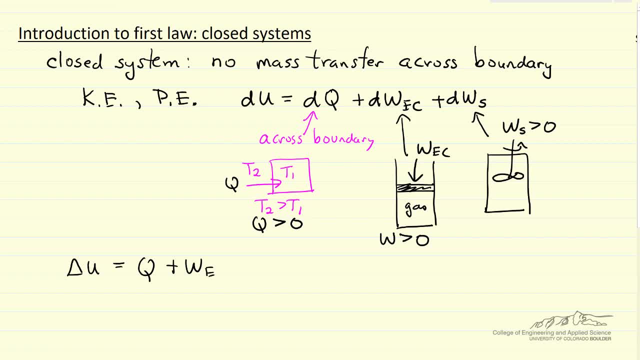 Q plus work for expansion, compression work, for shaft work and now this term, expansion compression work is minus integral pressure, external, In other words, when pushing down it's this pressure that determines the work for pushing down or if it's pushing. 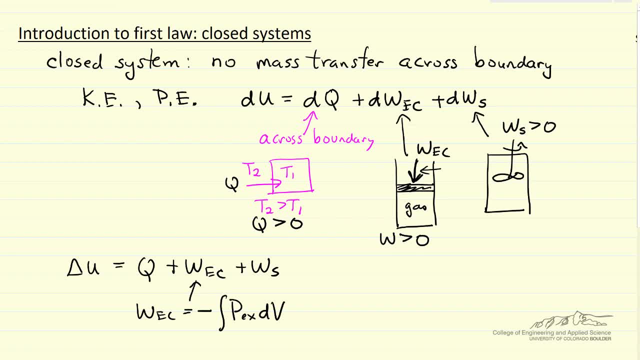 the gas is expanding and pushing up. The negative sign is here because if the volume decreases. so this were negative, then the work would be positive, and that's what we've looked at here. The work is positive if we're compressing a gas. 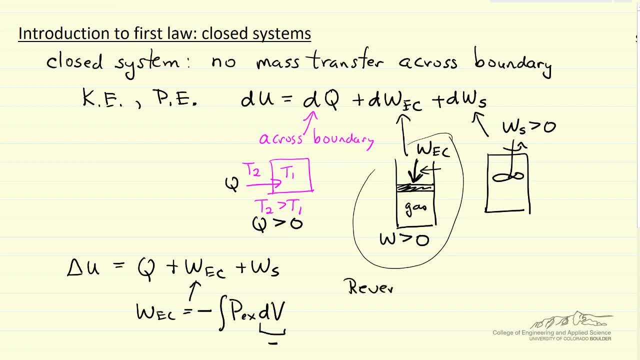 If it's reversible- and we'll talk elsewhere other screencasts what we mean by that- then this expansion, compression work is minus integral of the pressure of, for example, the gas inside the system. Only if it's reversible that we can use the pressure. 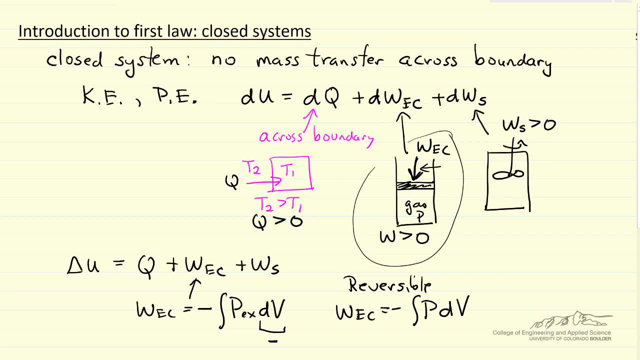 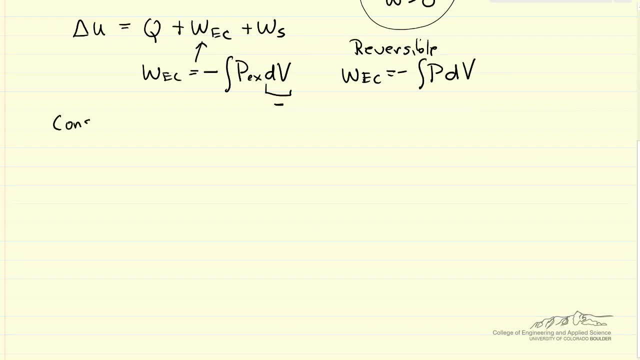 in here. otherwise it's external pressure that is used in our calculation of work. So one common one might be a constant pressure process and then delta U. again we're talking about a closed system. Q- constant pressure, we can bring it outside.